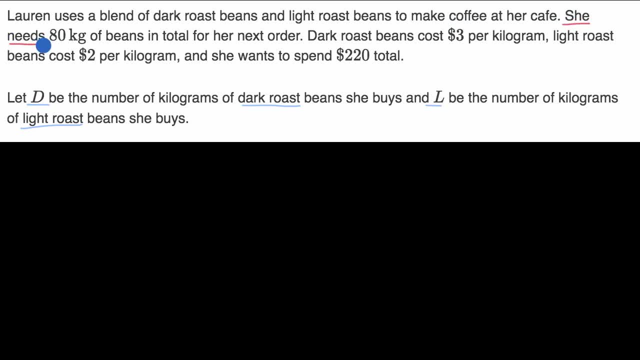 And then they tell us here: they say she needs 80 kilograms of beans in total. So what we could say is: hey, the number of kilograms of dark roast beans plus the number of kilograms of light roast beans needs to be equal to 80 kilograms. 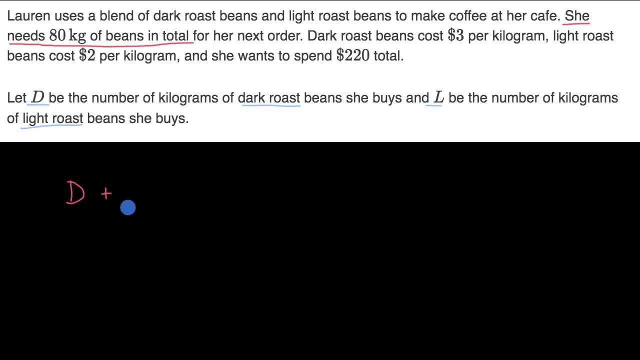 So the number of kilograms of dark roast beans plus the number of kilograms of light roast beans- I'm having trouble saying light roast beans- well, this what I just underlined here. it says it needs to be 80 kilograms in total. 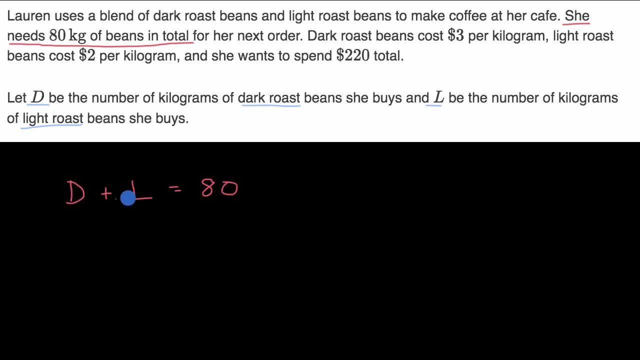 So that needs to be 80.. So this number of kilograms plus this number of kilograms is going to be equal to your total number of kilograms. All right, so I have one equation with two unknowns. Let's see if we can get another one. 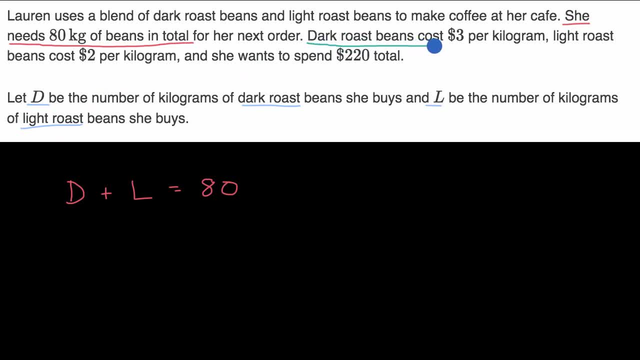 So next they say dark roast beans cost $3 per kilogram, Light roast beans cost $2 per kilogram, And she wants to spend $220 total. So what I just underlined in this aquamarine color we can set up another equation with. 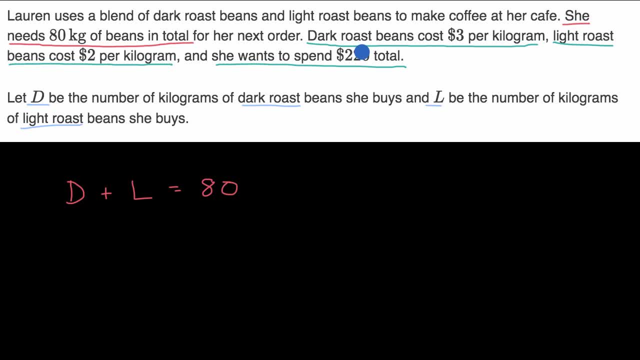 And if you haven't already set up your system of equations, you can do that here. You can set up your system of equations. See if you can now do that. See if you can set up the second equation. Pause the video, All right? well, the way to think about it is. 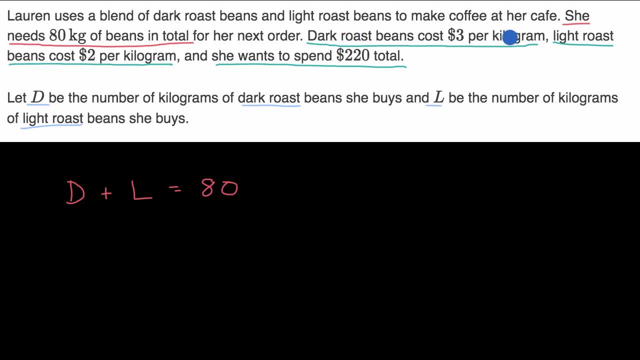 we just have to have an expression for how much does she spend on dark roast beans? how much does she spend on light roast beans? and then we need to add those two together and that needs to be equal to $220, because that's how much she wants to spend in total. 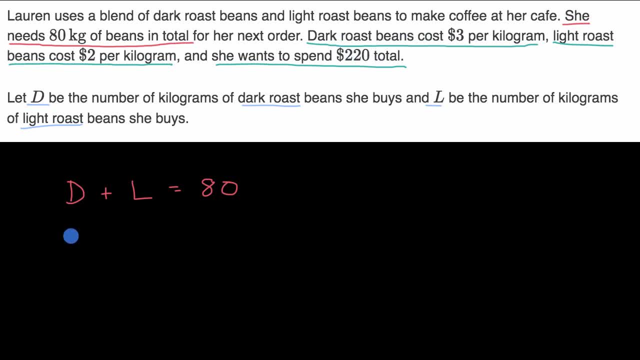 So how much does she spend on dark roast beans? Well, it's going to be the number of kilograms of dark roast beans that she buys, and it says that it costs $3 per kilogram. So we're going to multiply it by three. 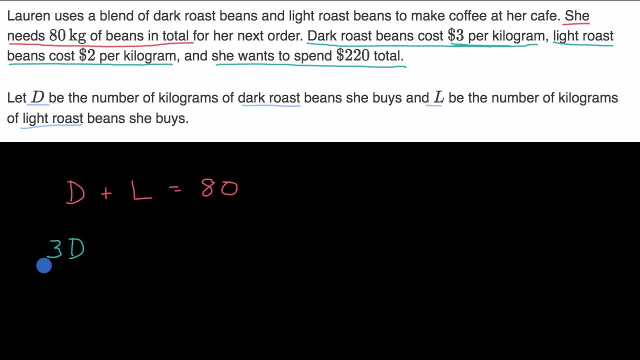 $3 per kilogram times the number of kilograms of dark roast beans. This is how much she spends on dark roast beans. And so how much is she going to spend on light roast beans? Well, she buys L kilograms of light roast beans. 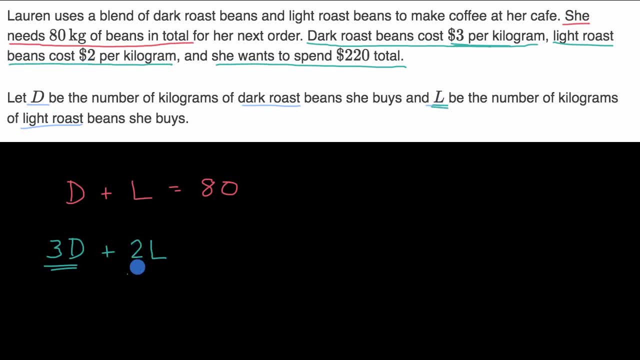 They told us that there And they cost $2 per kilogram. so $2 per kilogram times the number of kilograms, This is how much she spends on light roast beans. So you add how much she spends on dark roast to how much she spends on light roast.